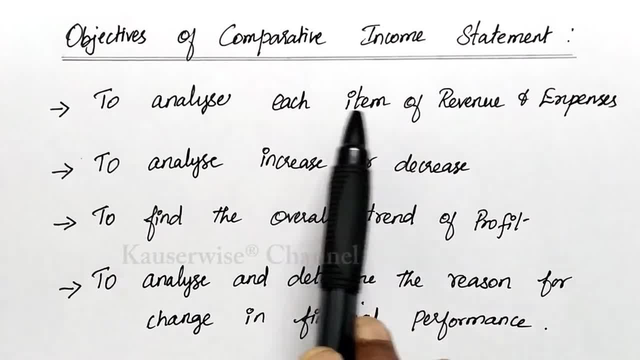 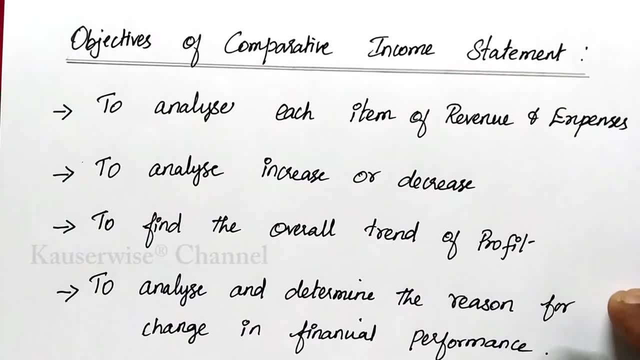 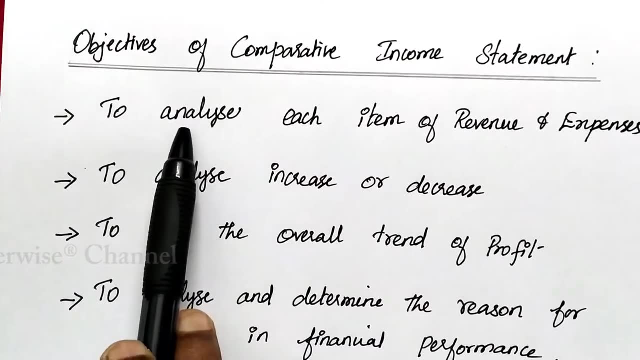 The first one is to analyze each and every item of revenue and expenses. Okay, see, in the income statement you can see the list of revenue and list of expenses. Okay, so, with the help of comparative income statement, you can able to analyze each and every item. 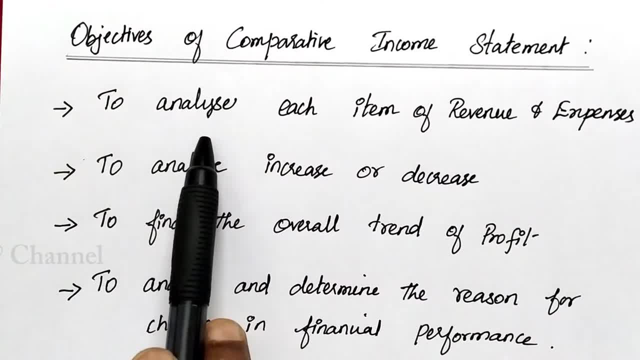 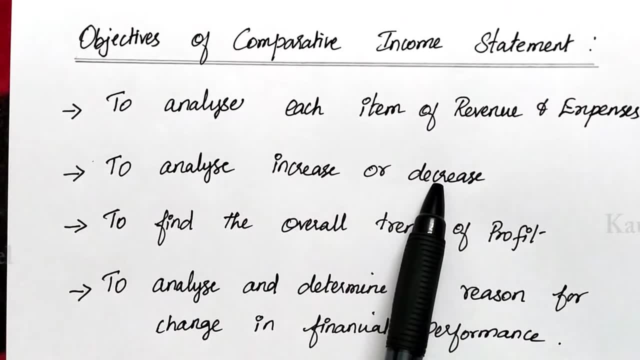 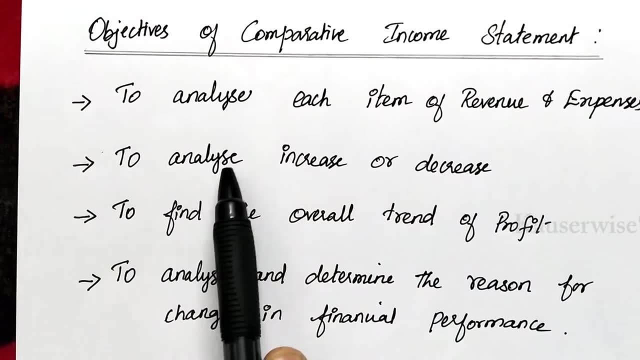 of revenue and expenses. Okay, is the main objective of comparative income statement. and the next one is to analyze increase or decrease. okay, either increase or decrease of each and every revenue as well as expenses that can be analyzed with the help of comparative income statement. and the next one is: you can 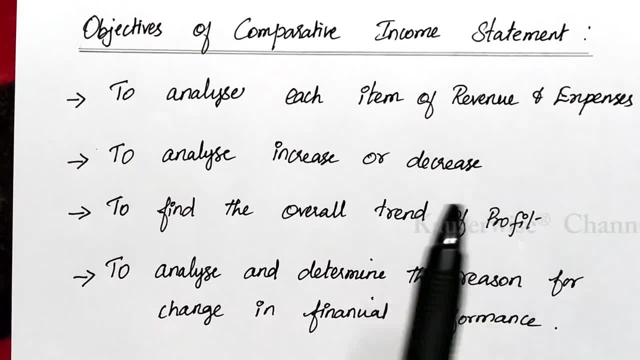 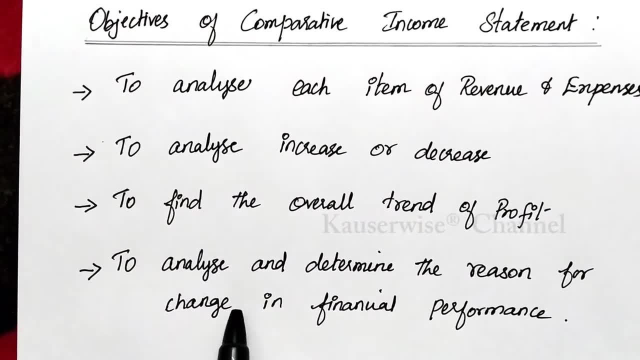 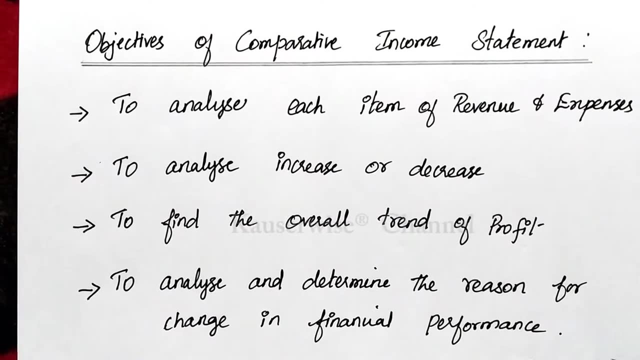 able to find out the overall trend of profit that can be identified with the help of the comparative income statement. and the last one is: you can able to analyze and determine the reason for change in financial performance. okay, so these are the various objectives of comparative income statement, or. 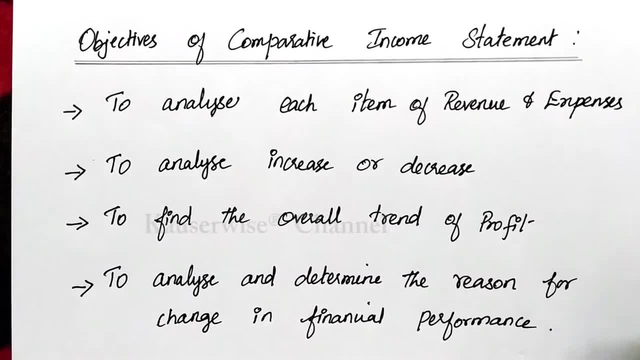 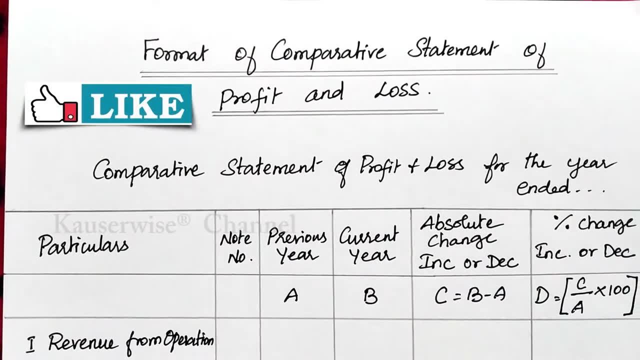 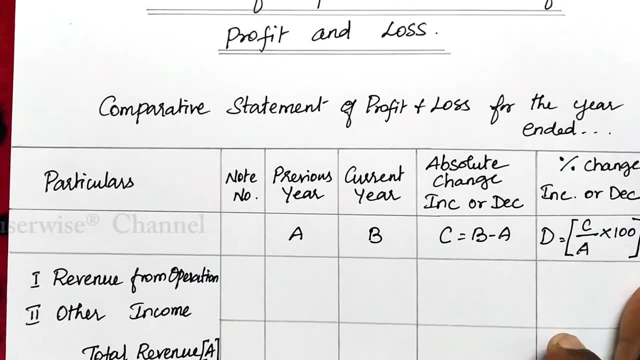 comparative statement of profit and loss. okay, now we are going to see the format for comparative income statement. then we will see the problem. see the format of comparative statement of profit and loss. okay, for the year ended two years, informations will be there. you see, here we have six columns. the first one, particulars, next one working note number. 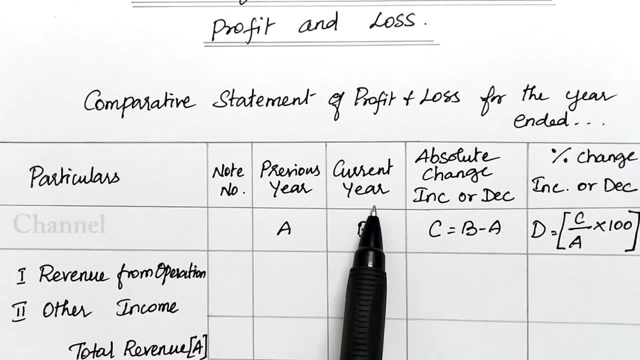 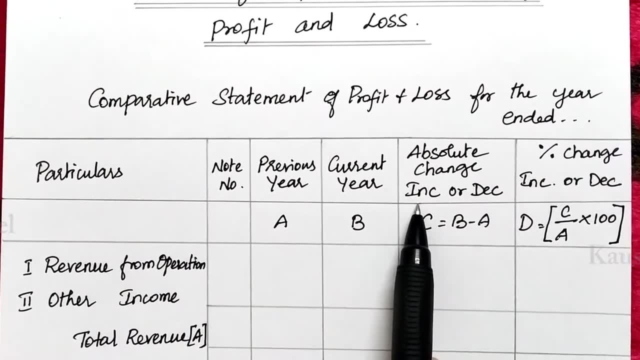 the next one previous year data and the next one current year data. okay, and the next one, absolute change. that is, when you compare these two informations, you will be getting either increase or decrease. the change will be there. this is called as absolute change. and the last one: 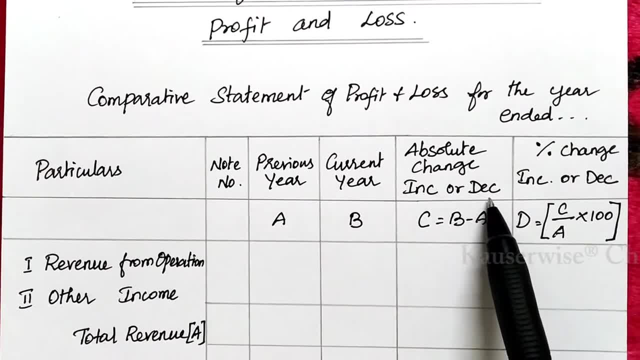 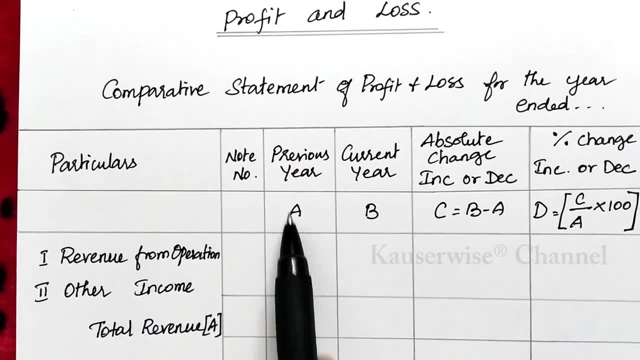 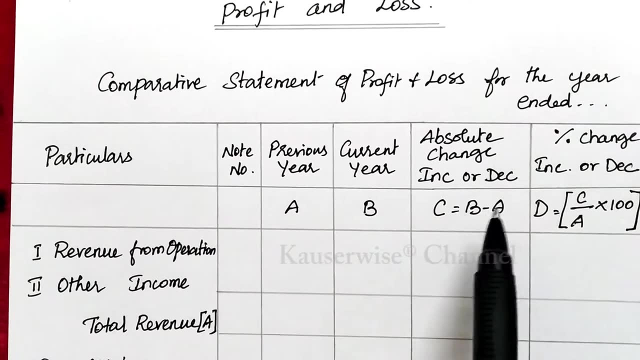 percentage change. okay, so after finding increase or decrease, that is absolute change. finally, you have to calculate the percentage. okay, with the help of the formula. okay, this one is: a, that is previous year data. b- current year data. then we need to find out: c, that is absolute change for that, b minus a current. 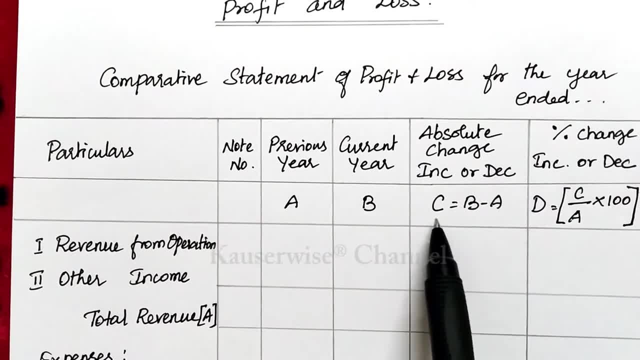 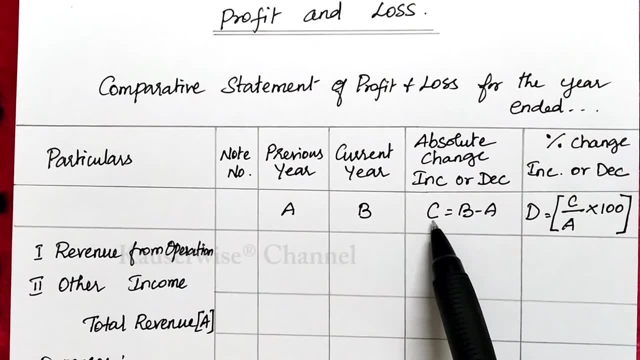 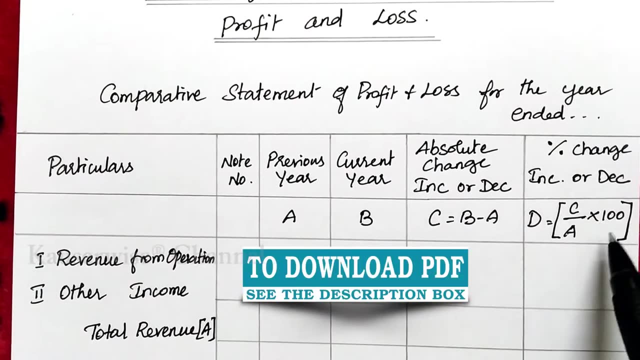 year data minus previous year data, you will be getting absolute change. then the percentage d is equal to c divided by a into 100 c for absolute change and divided by a for previous year data. so a, that is previous year data, is the base data. okay, so with that you can find out the percentage. 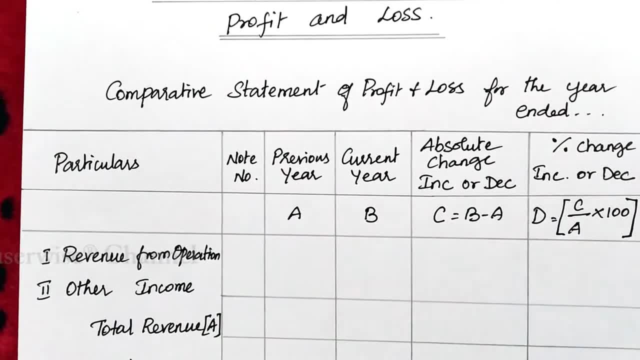 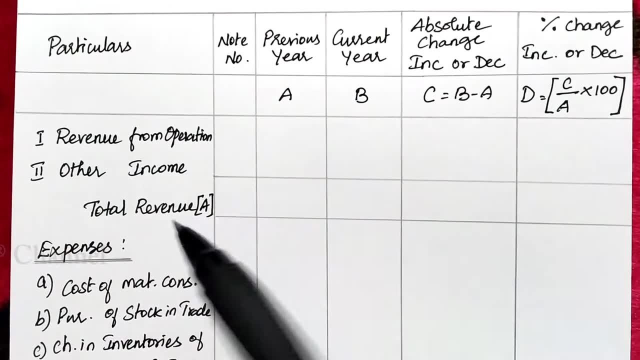 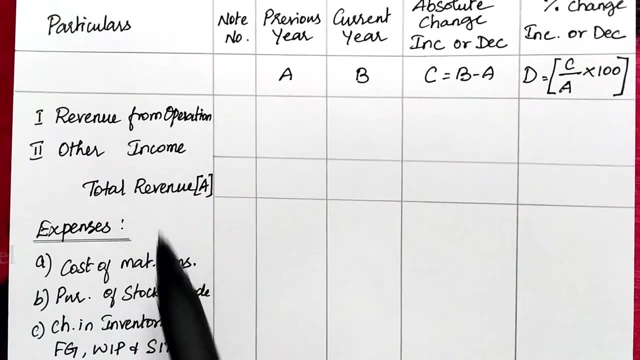 change. okay, this is the way to prepare comparative income statement. okay, now, under particulars, we'll be having total revenue and total expenses under total revenue. two things are there: revenue from operation and other revenue. these are the two components of revenue, okay, and the next one: expenses under expenses. we'll have different components, okay, the first one. 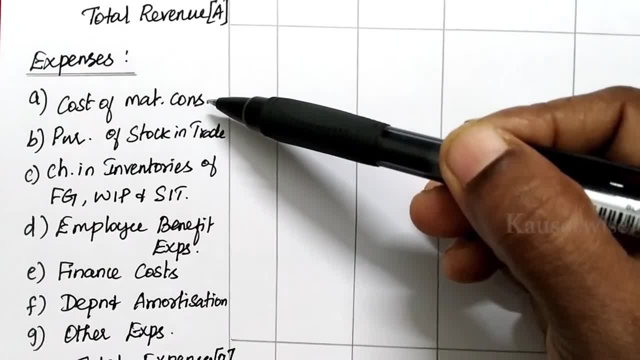 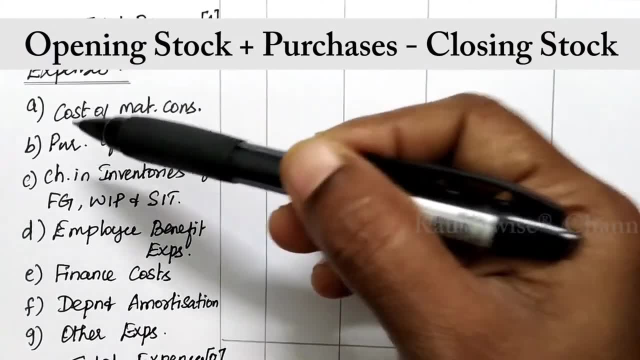 cost of living: okay. the second one: cost of living: okay. the third one cost of living: okay. cost of material consumed. there is a formula to find out cost of material consumed. that is a opening stock plus purchases, minus closing stock, you will be getting cost of material consumed. 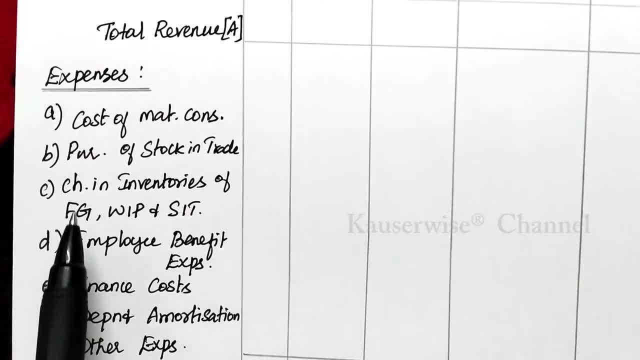 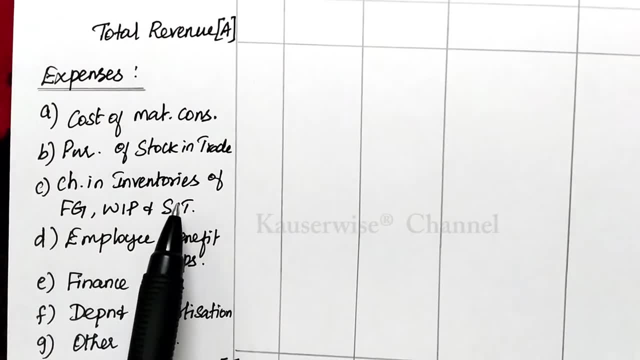 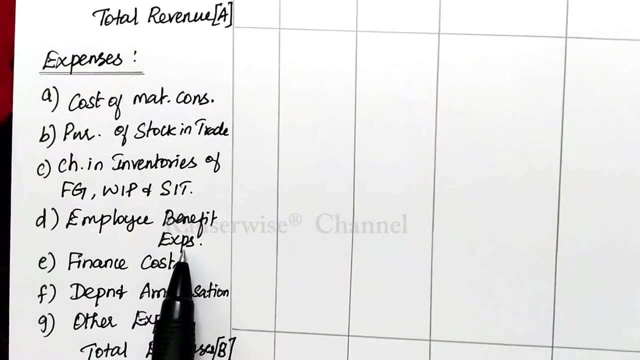 and the next one: purchase of stock in trade and then change in inventories of finished goods, work in progress or stock in trade. okay, if there is any opening and closing value, in that case you need to find out. change in inventories. and the next one: employee benefit expenses. 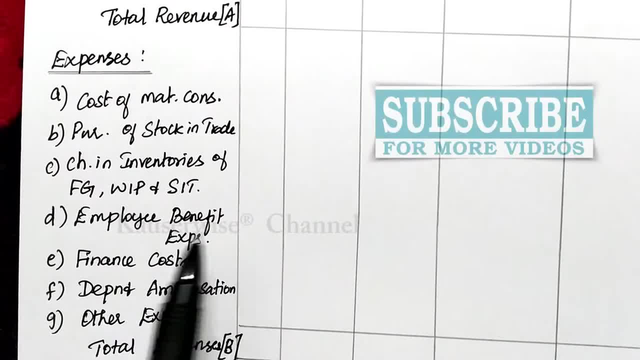 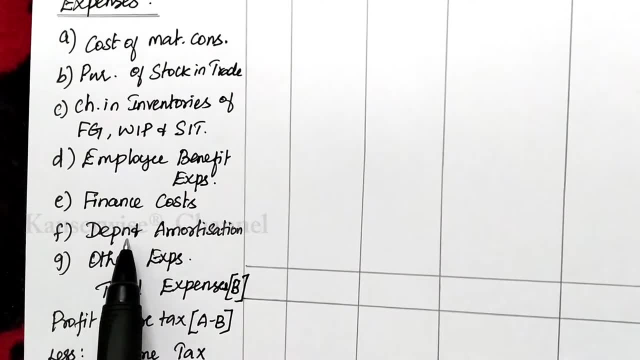 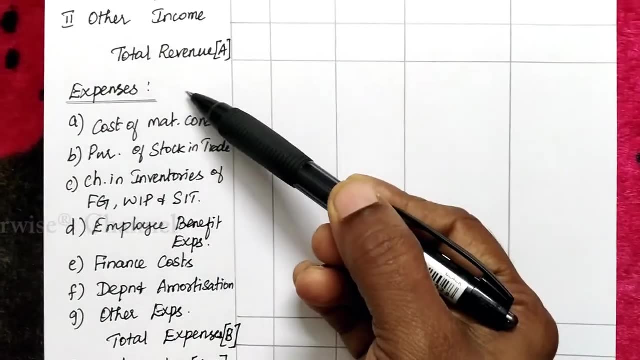 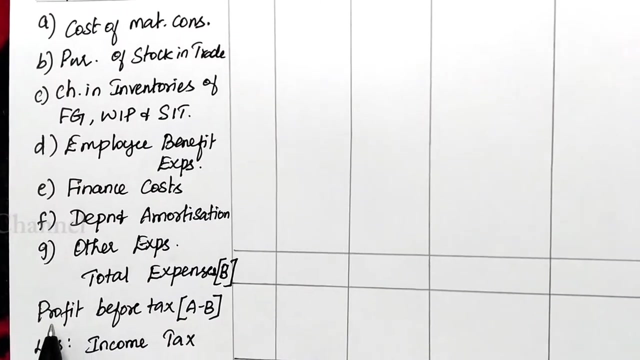 anything payable to employees or laborer- such things will be- comes under employee benefit expenses, and the next one finance cost and the next one depreciation and amortization and the last one other expenses. these are the various components of expenses. then you'll be getting total expense. after recording total revenue and total expense, then you need to calculate profit. 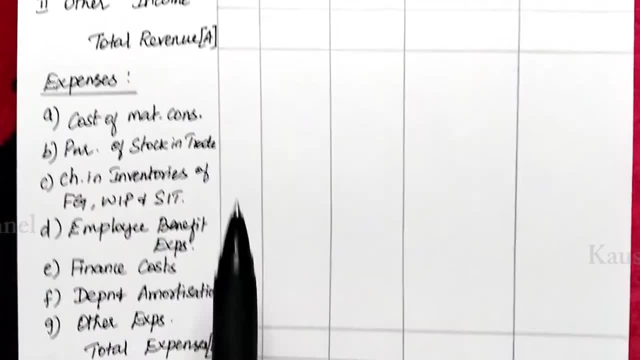 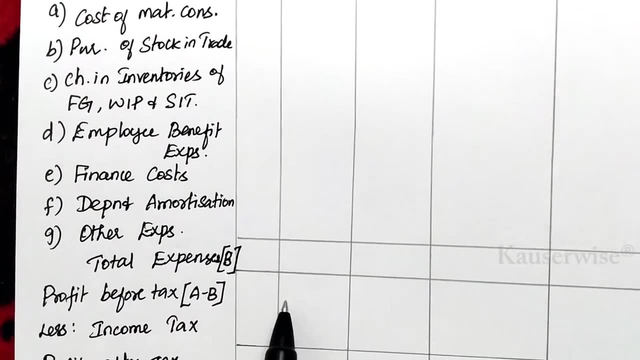 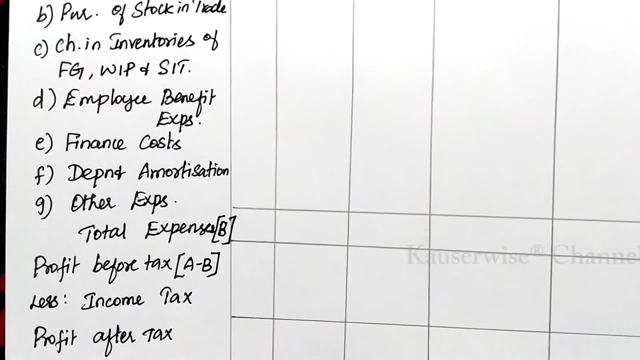 before tax. okay, that is a minus b. a denotes total revenue, b denotes total expenses. so revenue minus expense, you will be getting profit. if there is any information related to income tax that is 50, 40 percent like that, if such information is there, means then you have to subtract a income tax. then 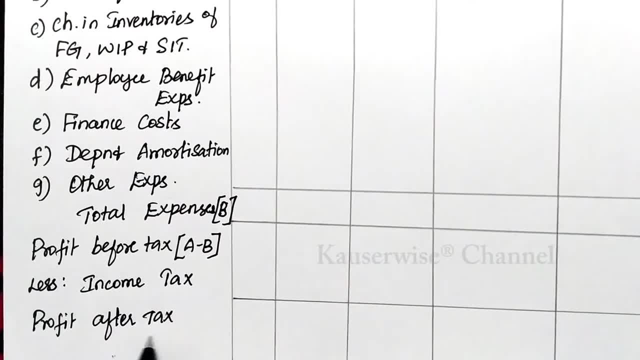 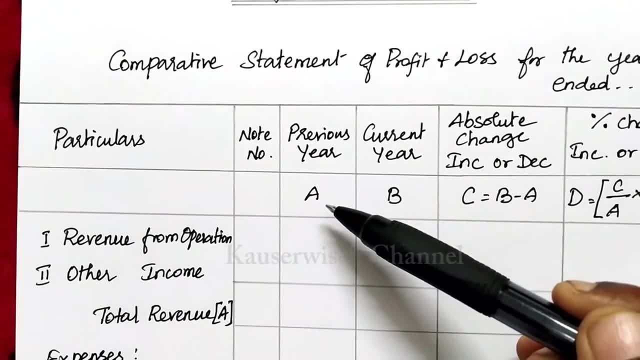 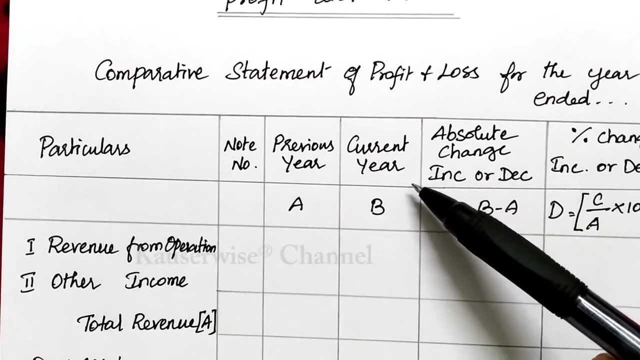 the profit. the remaining profit will be called as profit after tax. okay, this is the format of income statement. okay, now see in the previous year. okay, you have to enter all the data related to previous year. okay, under this column you have to enter the data related to current year. okay, current year information related to. 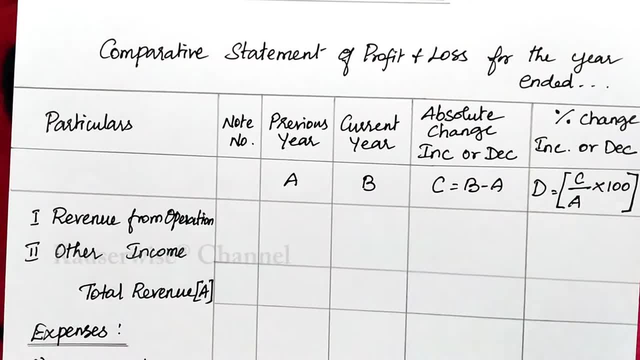 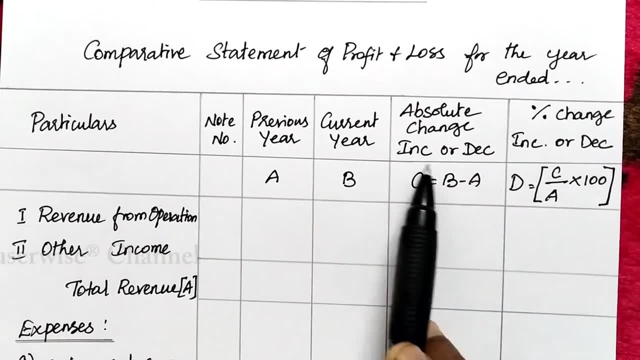 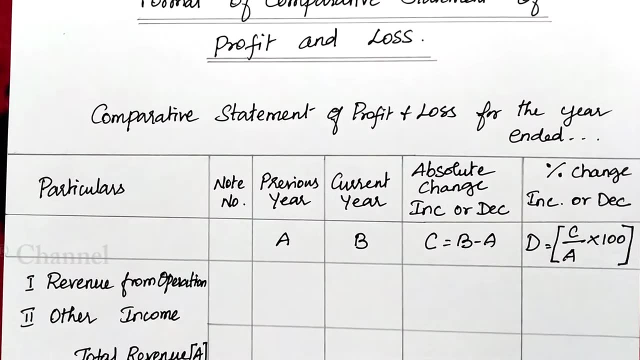 revenue and expenses, okay, and then, after recording previous year and current year information, then you can find out the absolute change, that is, increase or decrease. okay, the last one, percentage change. okay, you have to calculate the proportion that is percentage. for that you have to use the formula. 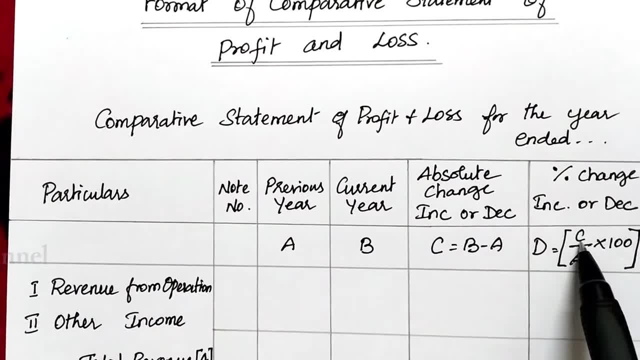 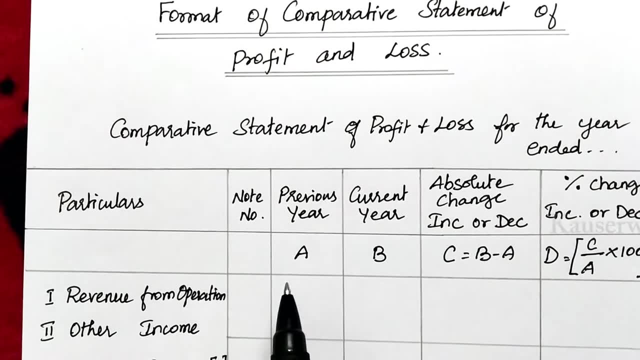 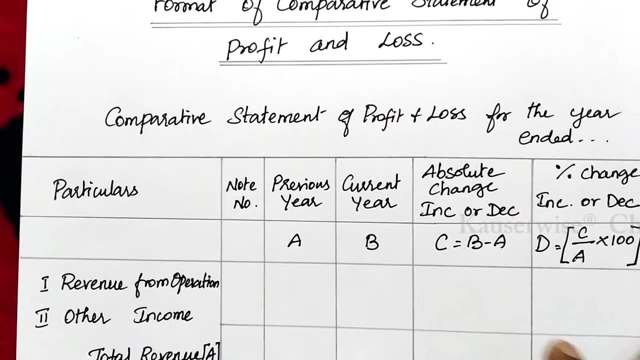 the formula is: c divided by a into 100. c represent absolute change. divided by a represent previous year information. okay, previous year data into 100, you'll be getting d. d means a percentage change. okay, so this is the format of comparative income statement. now we are going to see one. 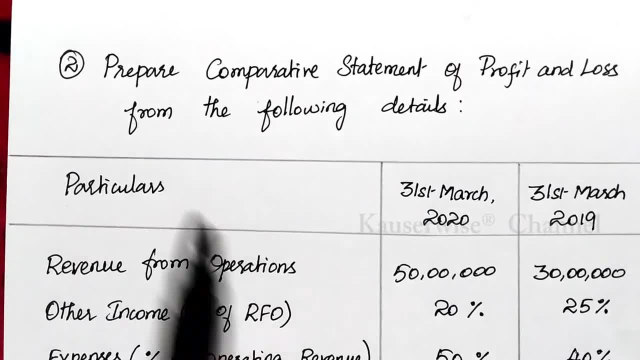 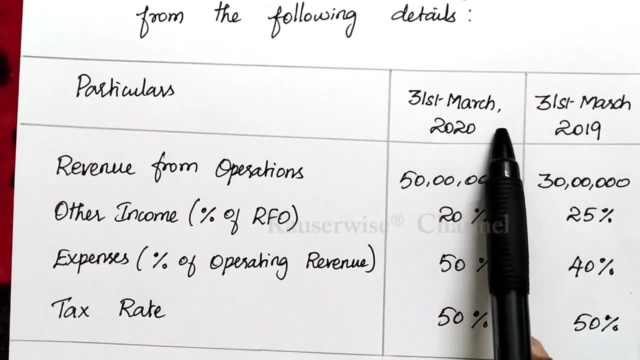 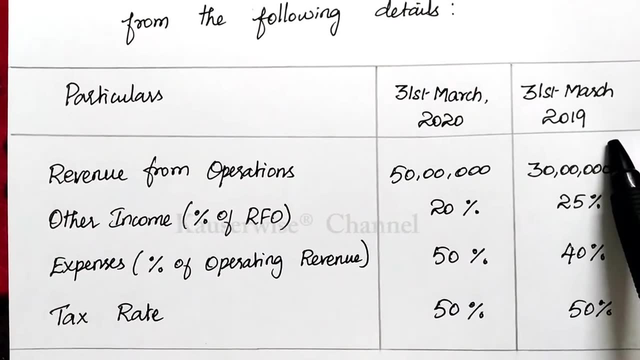 problem. to have a better understanding, see the problem, prepare comparative statement of profit and loss from the following details. so, as you see here there are some initial Illuminati細 topped letters, okay, which represent the percentage of profit. have taken kind of the ratio of market to market ratio, okay, so then, 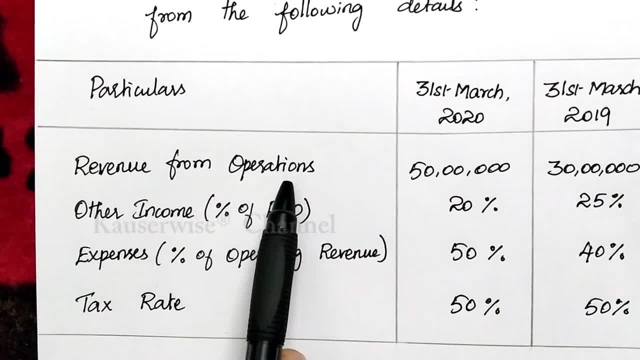 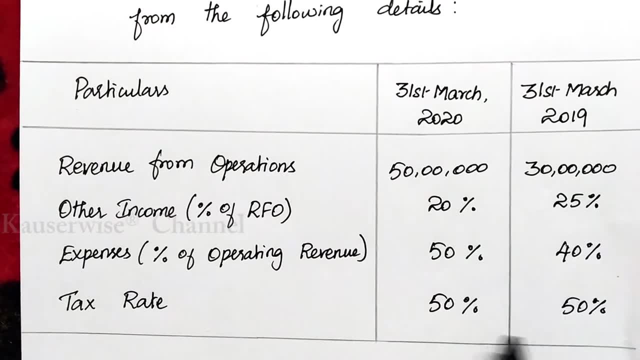 on this data. okay, as you can see here there's just카, respectively out group bkmera 1: limit the proportion and see how many indicators there are. so we are taking that icon which part in the report? okay, we're going to need one indicator in this report, okay, and then we give you this: 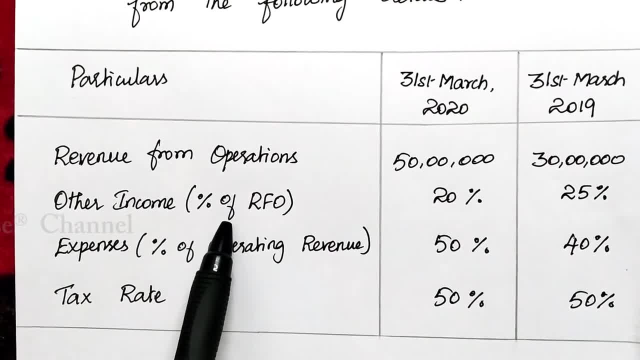 particular data, empty sum data. so beauty text, pretty above or kaku, and then then another asset: okay, good. so another result: equity is the property one plus this particular four, also given in the proportion, That is, percentage of revenue from operation, 20% of revenue from. 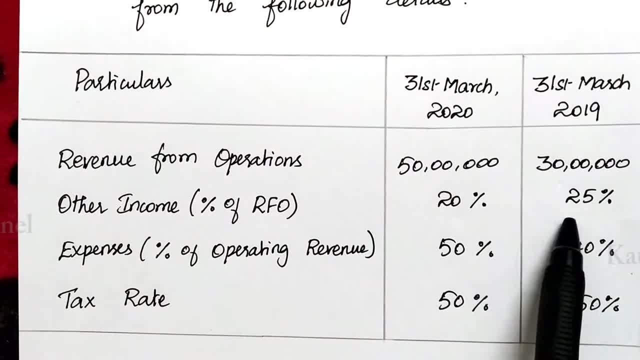 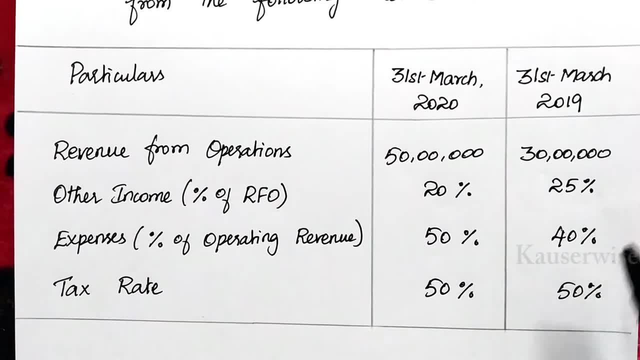 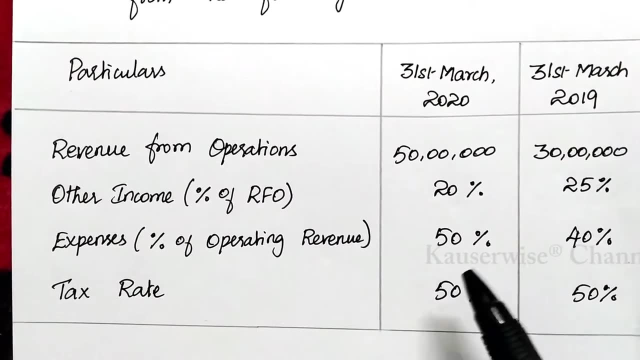 operation is the other income for the current year. In the same way, 25% of revenue from operation is the other income for previous year, Okay, And the next one, expenses. So expenses also given as percentage Percentage of operating revenue, Okay. So here, 50% of 50 lakhs is expense. 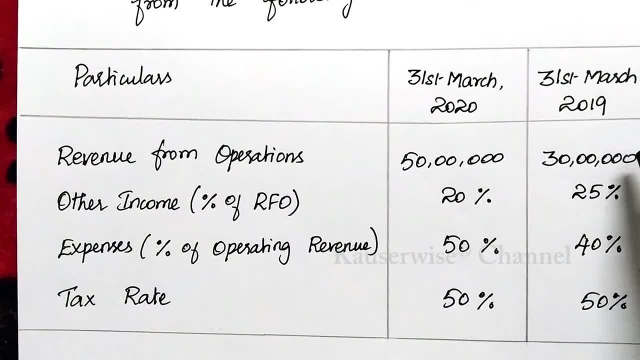 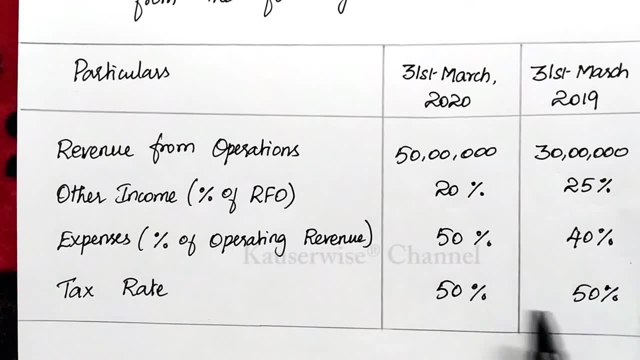 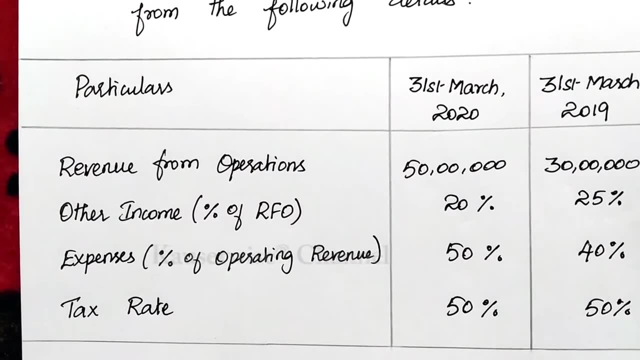 for the current year. In the same way, 40% of revenue from operation is the expense for the previous year. The next one: tax rate: 50%, 50%. Okay, With this information, they ask you to prepare comparative income statement. Now let us see the solution. See the solution of comparative. 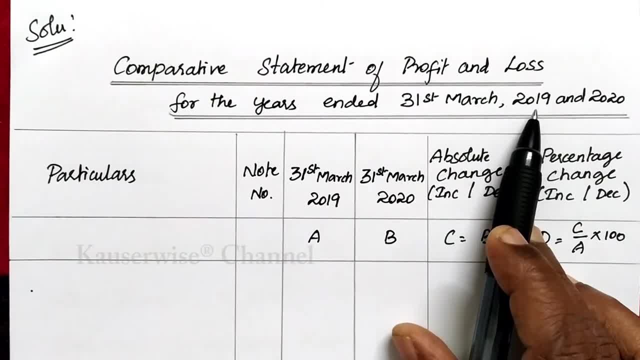 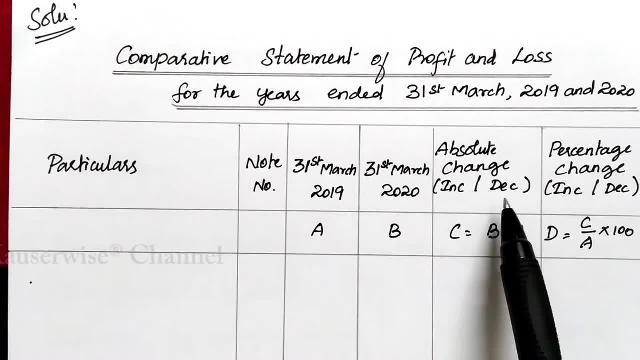 statement of profit and loss account for the year ended 2019 and 2020.. Okay, Particulars note number 2019, 2020.. Absolut change and percentage change: Okay, And the particulars. the first item will be: 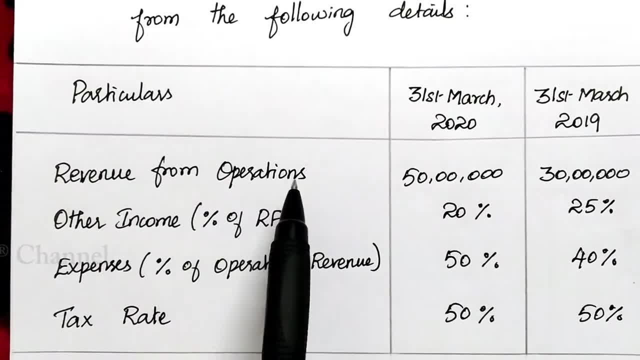 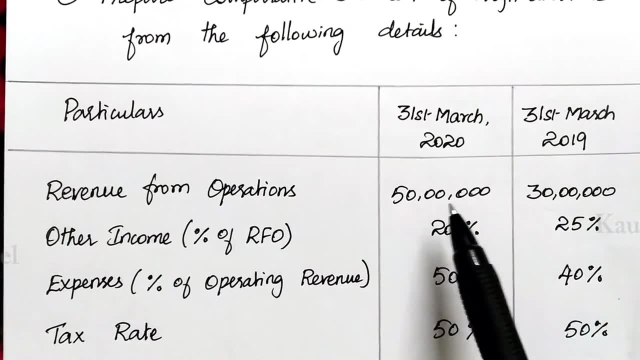 revenue from operation. See the problem. revenue from operation: previous year: 30 lakhs. current year: 50 lakhs. Okay, First you have to enter previous year, then you have to enter current year. Okay, See the solution. We have entered. revenue from operation previous year: 30 lakhs. 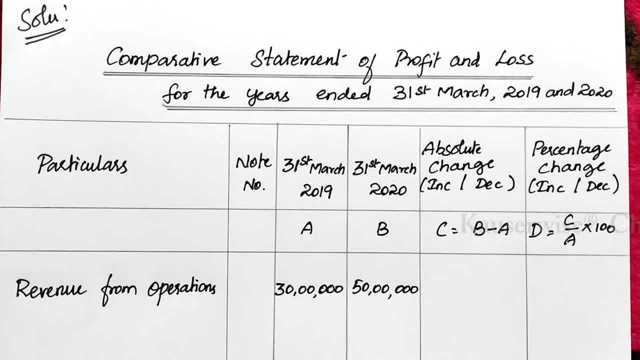 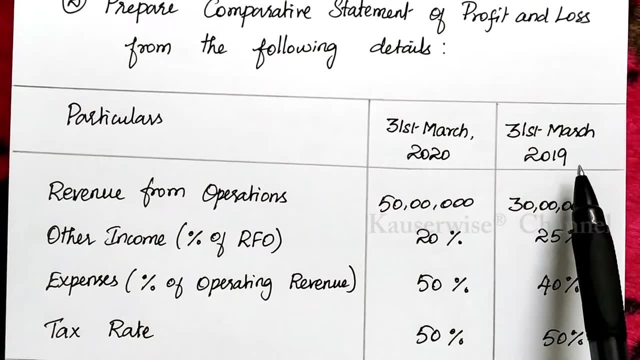 current year: 50 lakhs. Okay, The next one is other income. See the problem. See other income: 20%. 25% of 30 lakhs is the other income for the previous year. Okay, for the current year: 20% of 50 lakhs. 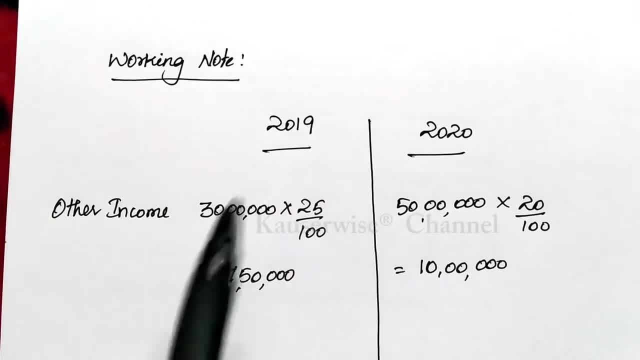 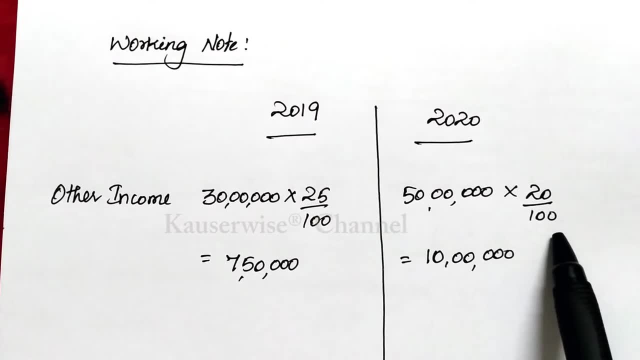 Okay, see the working note. Other income for the previous year: 30 lakhs into 25%, is 7,50,000.. For the current year, 50 lakhs into 20%, that is 10 lakhs. Okay, enter this in the comparative statement. 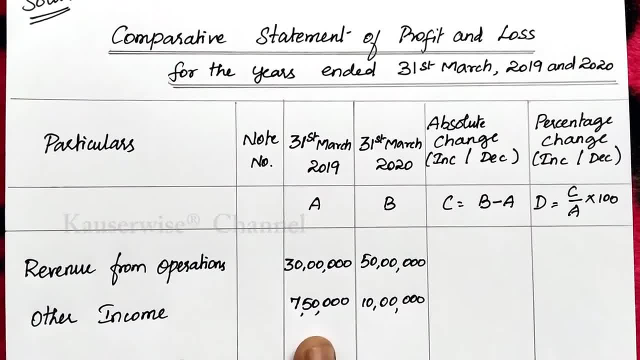 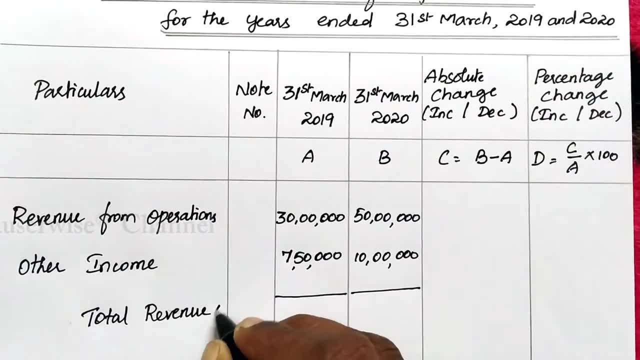 See the solution. We have entered other income: Okay, 7,50,000 and 10 lakhs. Now get the total. This is total revenue. That is A Okay 3 lakhs plus 7,50,000, 37,50,000.. 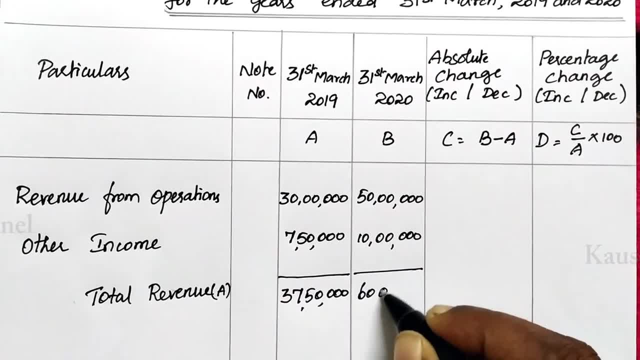 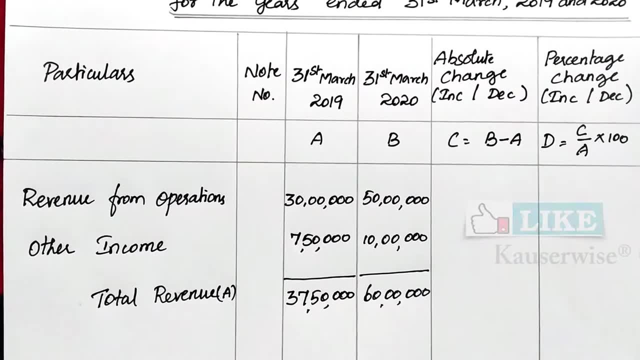 50 lakhs plus 10 lakhs, 60 lakhs. This is the total revenue. Okay, now we need to enter expenses. Okay, see the problem. See, expense is also given in the proportion, That is, percentage of. 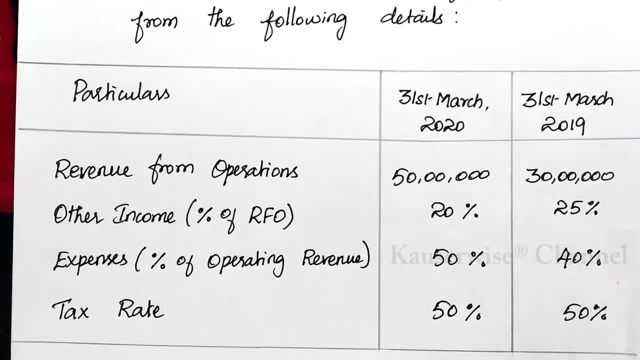 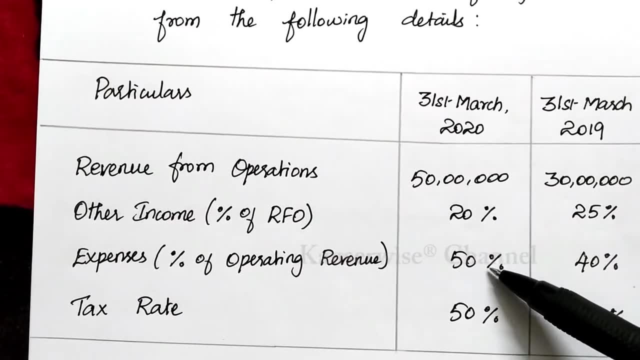 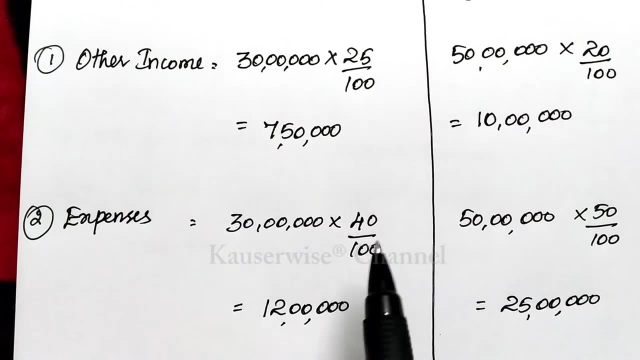 That is revenue from operation. See for the previous year, 40% of revenue is the expenses And for the current year, 50% of the revenue from operation is the expenses. Okay, see the working note. For the previous year, expense 40% of 30 lakhs. 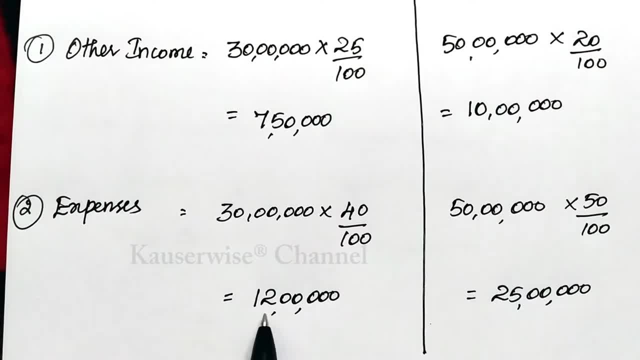 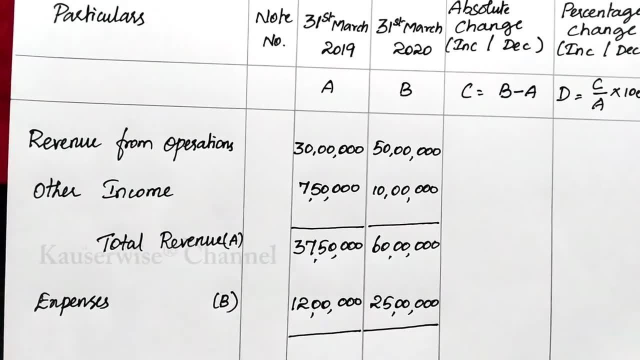 For the current year: 50% of 50 lakhs. Okay. for the previous year, 12 lakhs. For the current year, 25 lakhs. Now enter these values in the statement. See the solution. We have entered expenses for the previous year and current year. 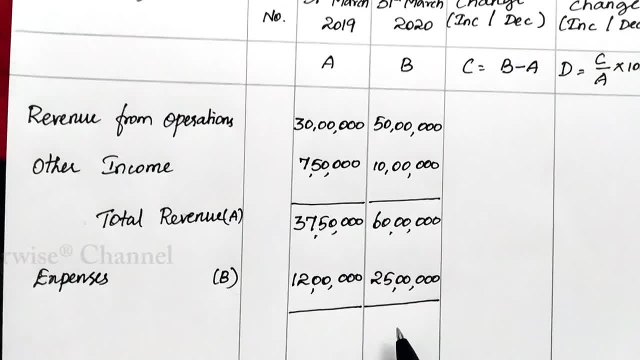 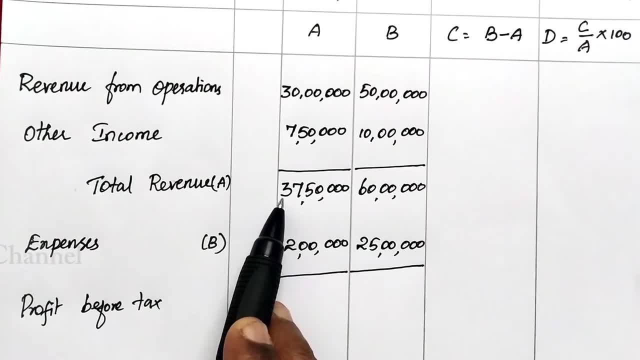 So previous year 12 lakhs, Current year 25 lakhs. Okay, so now we can find out the profit before tax. Okay, see, profit before tax. That is, total revenue minus total expense is equal to profit. 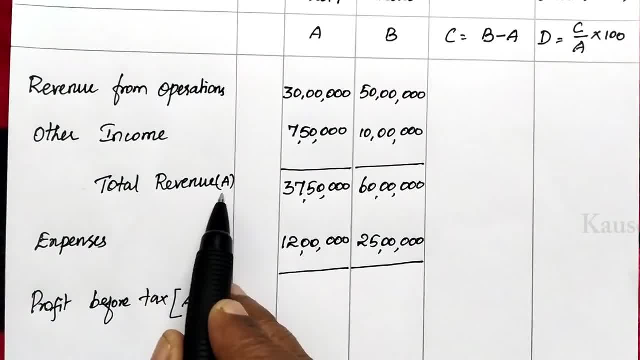 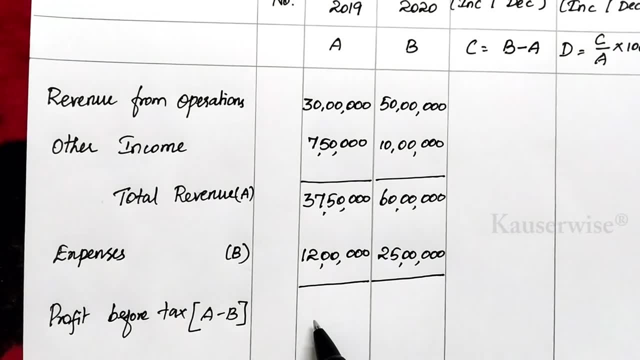 That is A minus B. A is total revenue, B is total expense. Okay, so, 37 lakhs, 50,000 minus 12 lakhs, You will be getting Profit before tax. In the same way for the current year: 60 lakhs minus 25 lakhs. 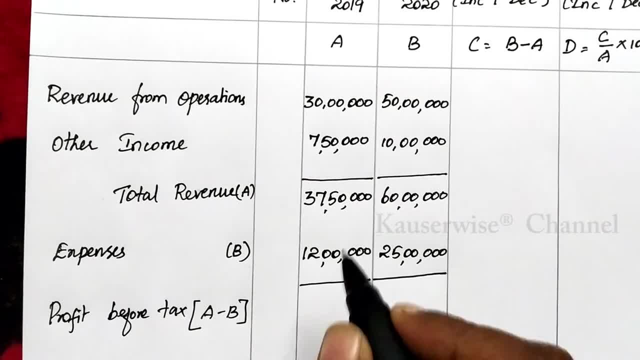 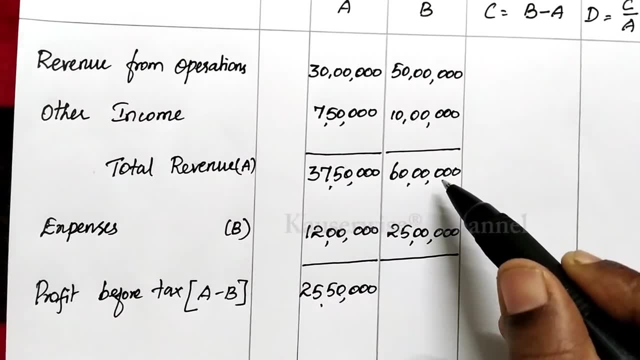 You will be getting profit before tax for the current year. Now just enter the value 25 lakhs- 50,000.. Okay, for the current year, 60 lakhs minus 25 lakhs, You will be getting 35 lakhs. 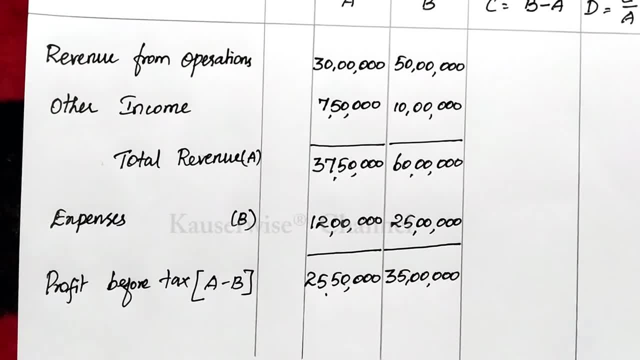 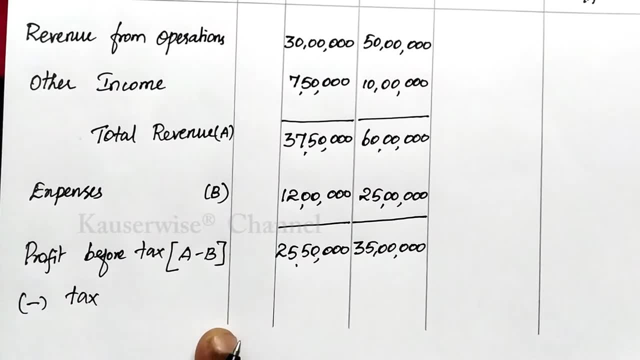 This is the profit before tax. Okay, now, in order to find out profit after tax, we need to subtract tax. Okay for tax. see the problem. See the problem. The tax rate is 50% and 50% for both the years. 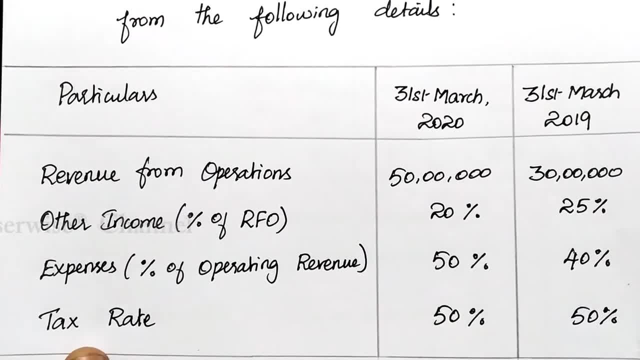 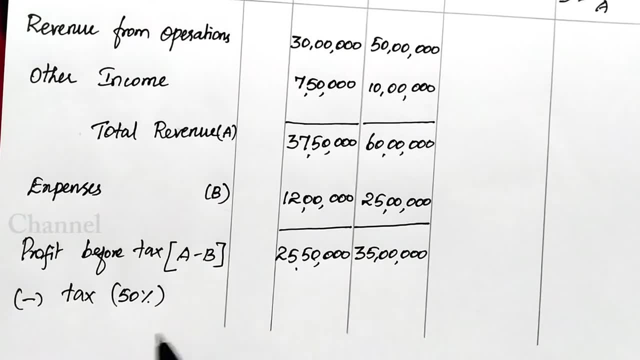 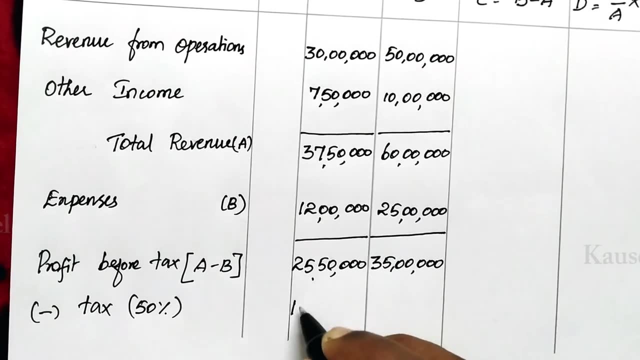 Okay, now calculate 50% of profit as tax. See the solution. The next one: subtract tax. That is 50% of 25 lakhs 50,000 and 50% of 35 lakhs. Okay, for the previous year, 50% of 25 lakhs 50,000 is 12 lakhs 75,000.. 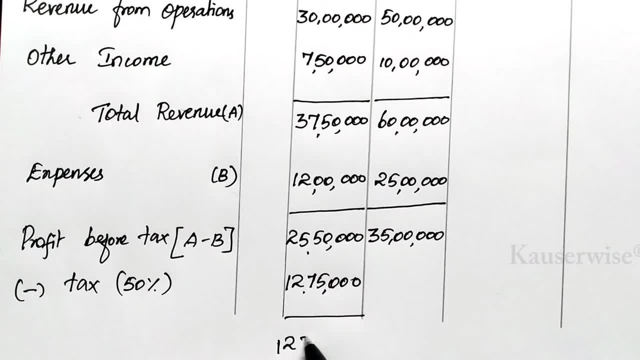 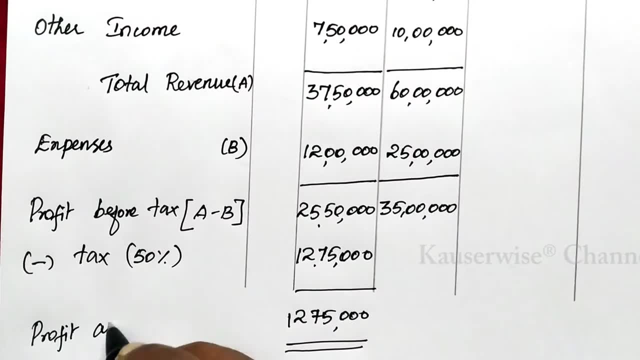 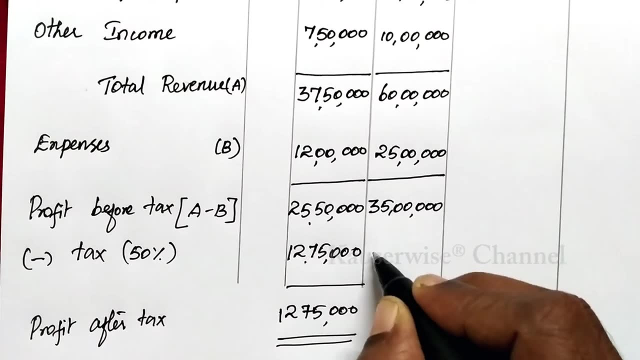 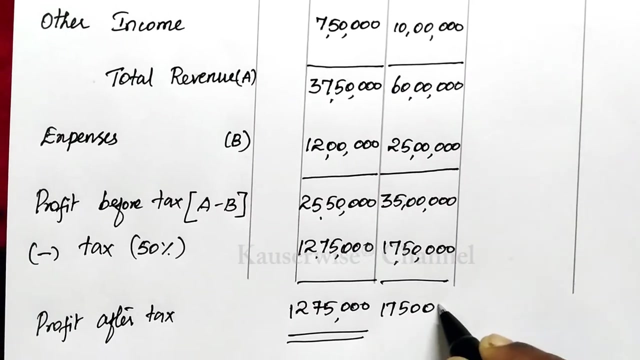 So the remaining 50% is That is profit after tax. Okay, In the same way for the current year, 35 lakhs into 50%- 17,50,000.. Tax balance: 50%- 17,50,000 is the profit after tax. 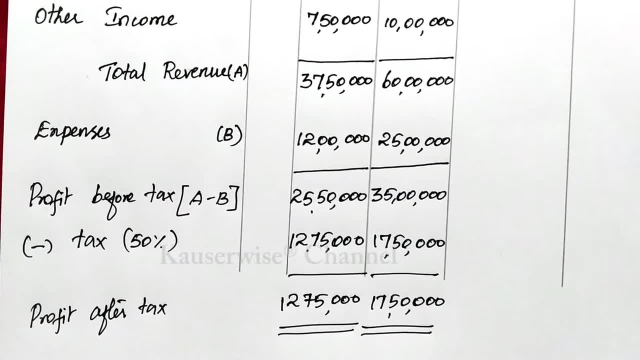 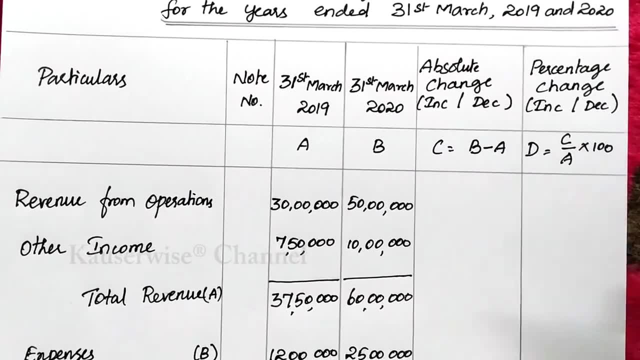 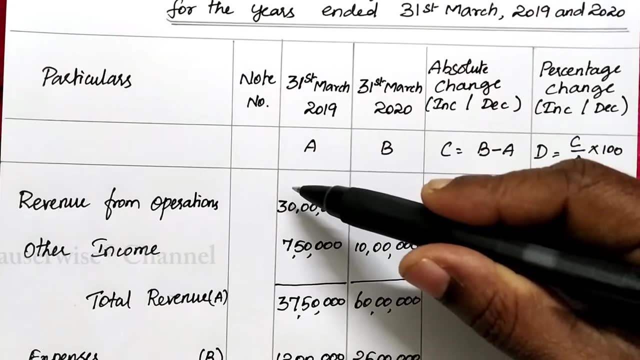 Okay, so we have got the profit after tax. Okay, for previous year And current year. Now the next calculation will be absolute change. We need to find the difference That is either increase or decrease. That can be calculated by comparing current year information with the previous year information. 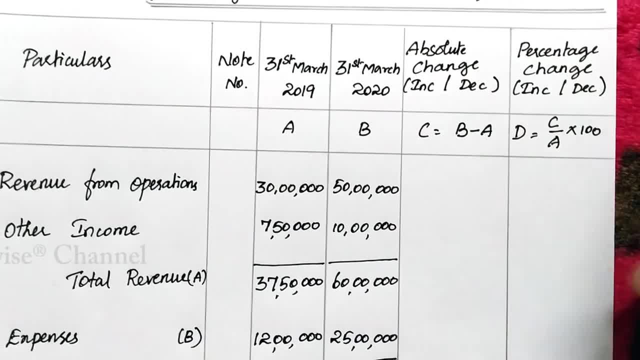 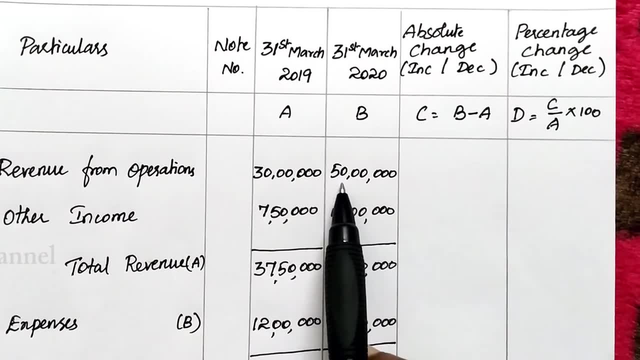 That is B minus A. You need to find, or you need to compare each and every item of the income statement. Okay, see the first item. The current year revenue is 50 lakhs. Previous year revenue, 30 lakhs, 50 minus 30.. 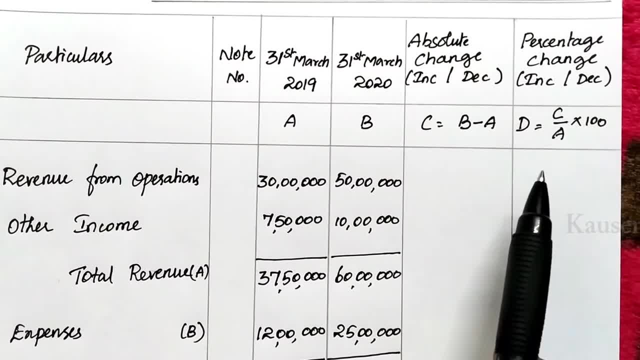 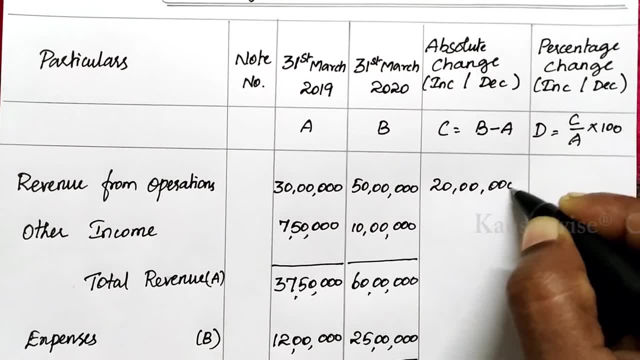 20.. That is the absolute change. That is increase, Positive change That you have to enter in this column 50 minus 30,, 20 lakhs. It's a positive increase. Okay. In the same way for the next item is 10 lakhs minus 7 lakhs- 50,000. 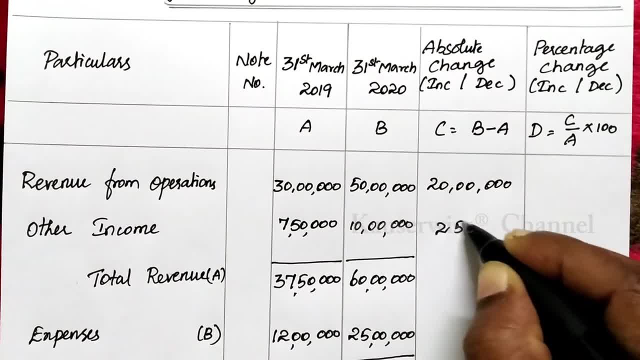 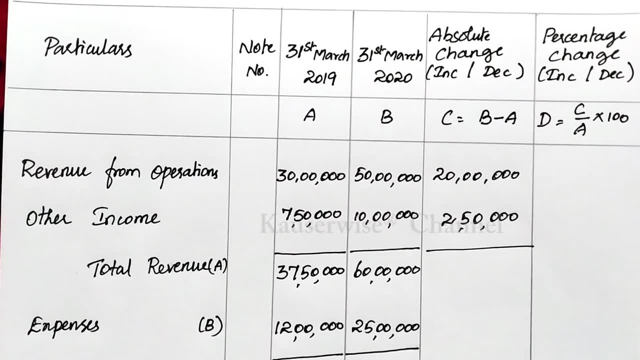 2 lakhs 50.. This is also increase Positive. So enter here: 2 lakhs 50,000.. In the same way, you have to compare each and every item in the horizontal format. Okay, See. 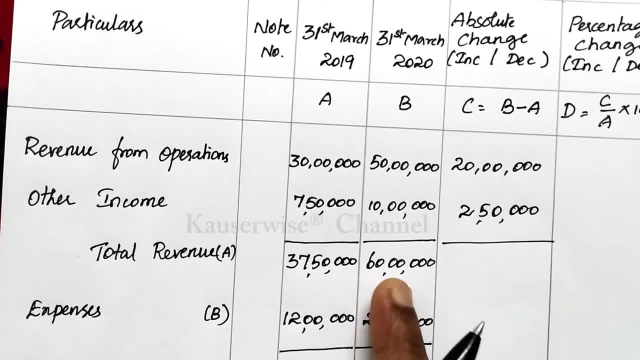 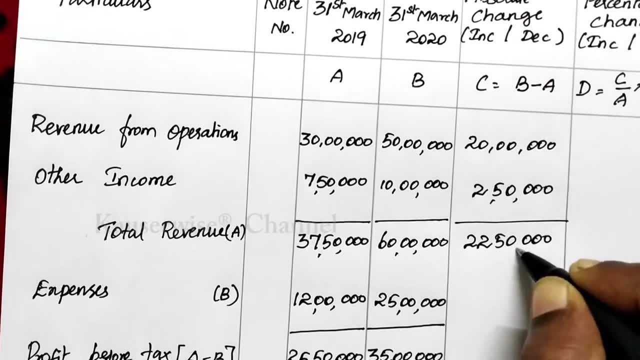 The next one: 60 lakhs minus 37 lakhs, 50,000.. Here also increase Positive value. Okay, How much? 22 lakhs, 50,000.. The next value: 25 lakhs minus 12 lakhs. 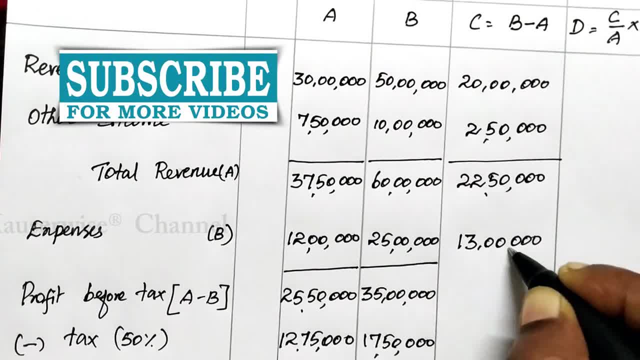 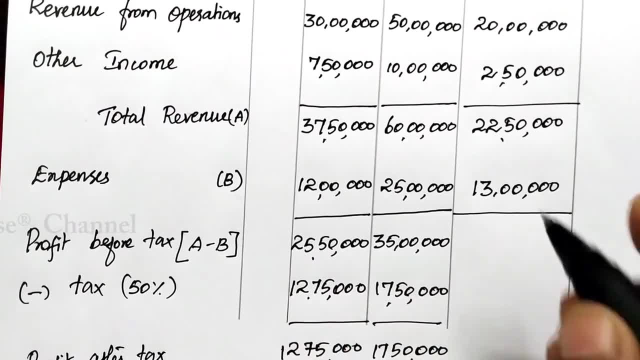 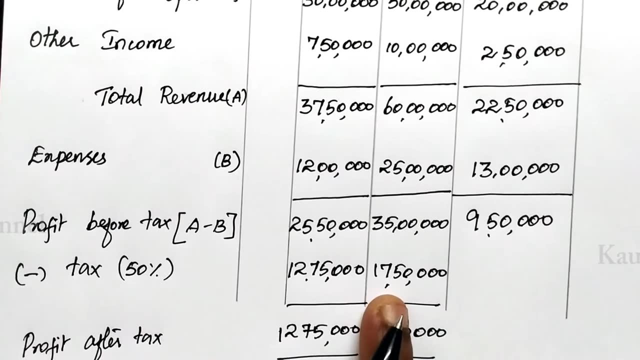 Here also positive value: 13 lakhs Increase. Next one: 35 lakhs minus 25 lakhs 50,000.. Here also increase Positive value: 9 lakhs 50,000.. And the next one: 17 lakhs 50,000 minus 12 lakhs 75,000.. 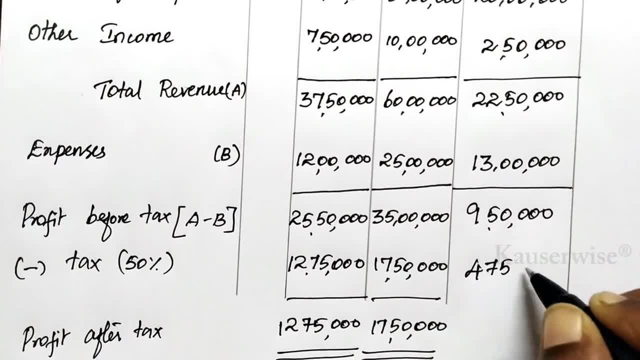 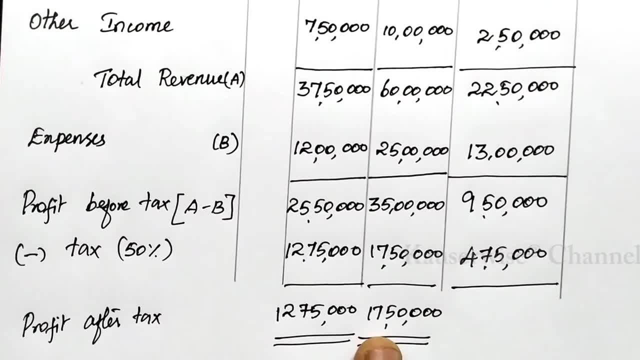 Here also positive value: How much Increase? 4 lakhs 75,000.. And finally you have to compare profit also: 17 lakhs 50,000 minus 12 lakhs 75,000.. Difference: 4 lakhs 75,000 increased. 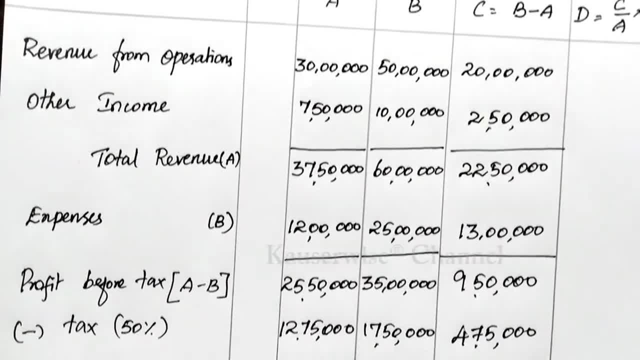 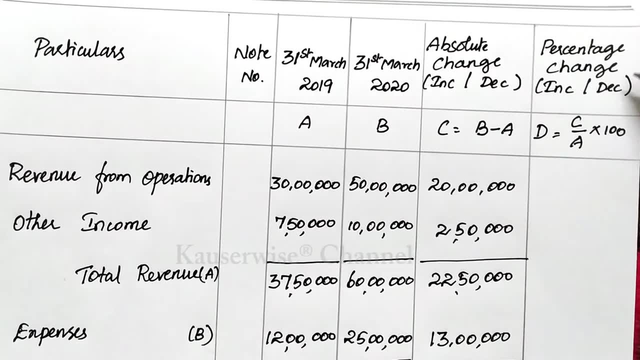 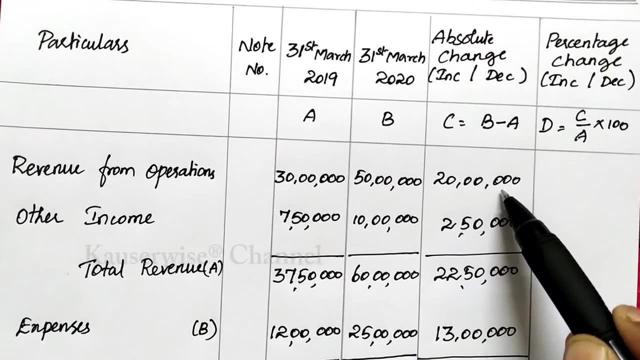 Okay, So this is the way to calculate absolute change. Okay, Simply comparing current year data with the previous year data, The last calculation is percentage change. For that you have to apply the formula to find out the percentage change. The formula is absolute change divided by base year. 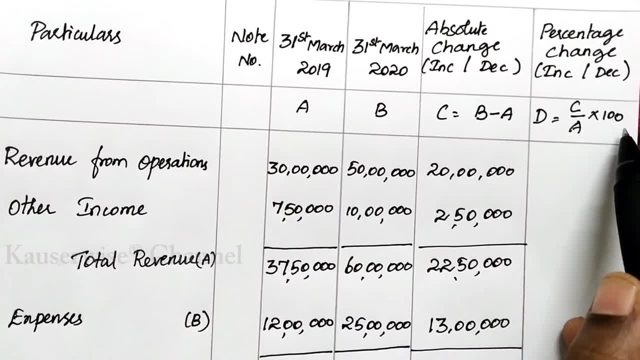 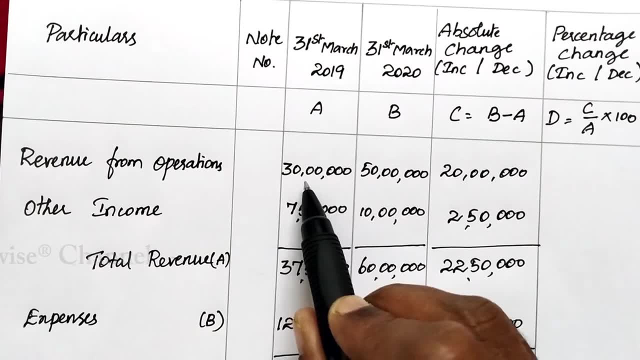 That is the previous year, is the base year. A Okay Into 100, you will be getting percentage change For the first one: 20 lakhs divided by 30 lakhs into 100.. 66.66. Okay. 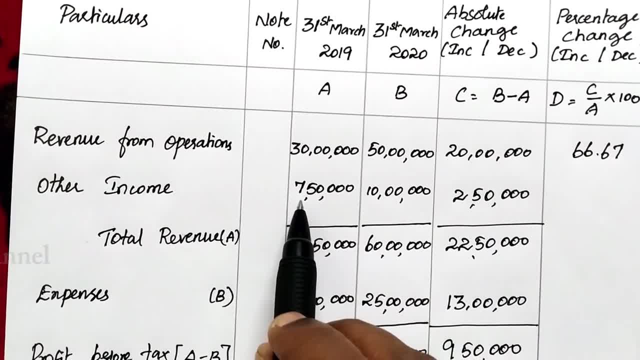 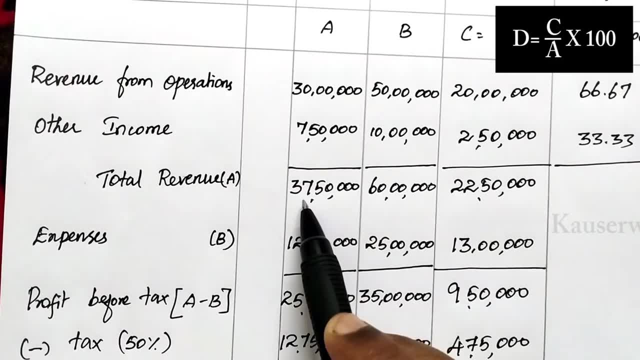 The next one: 2 lakhs 50 divided by 7 lakhs 50 into 100.. 33.33.. In the same way, the next value: 22 lakhs 50,000 divided by 37 lakhs 50,000..